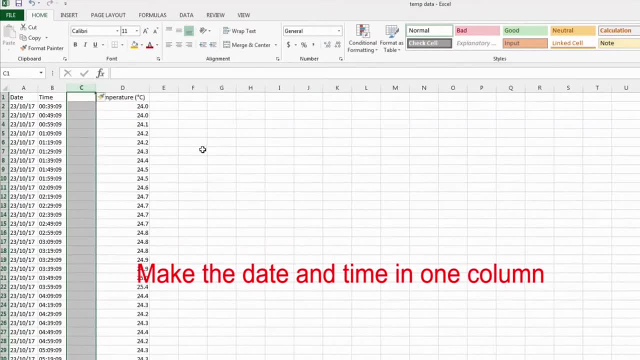 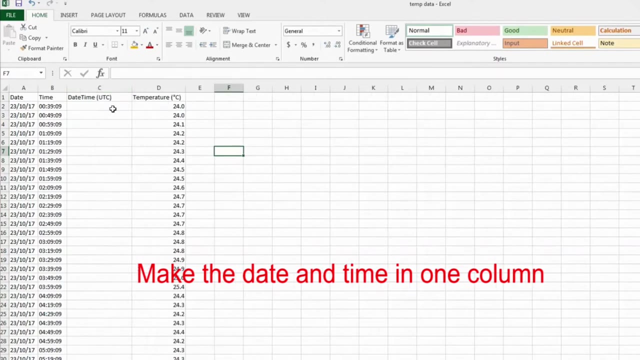 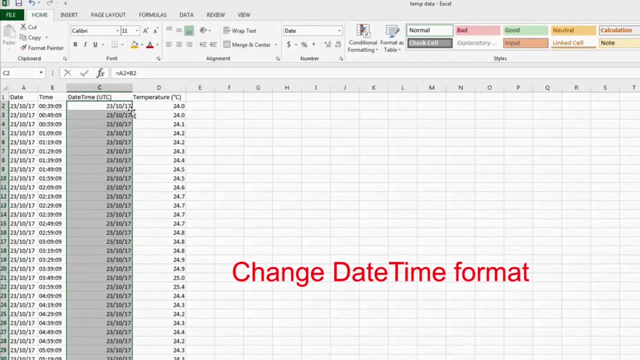 to create a new column. We can easily combine date and time using formula Date time And use the formula. C2 equals A2 plus B2. And double-click to apply the formula to the whole column. Remember to check date-time format, Because loggers have different formats for displaying. 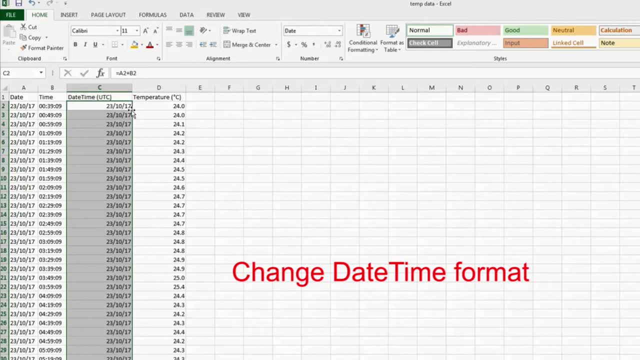 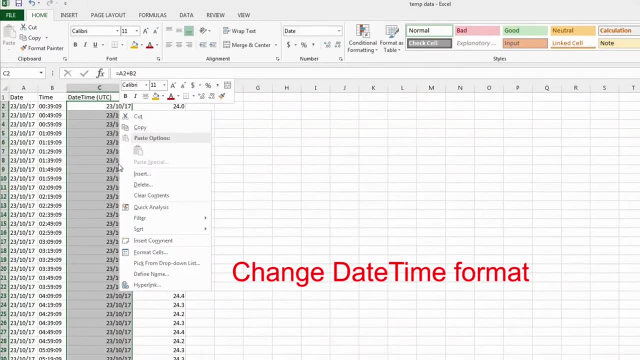 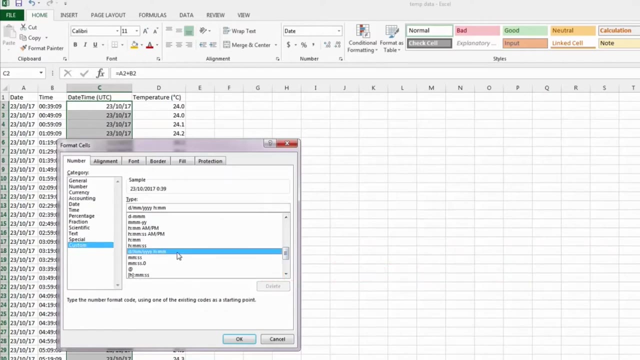 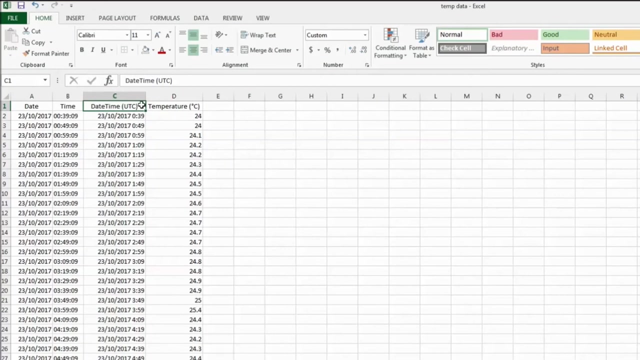 date and time, while Excel requires a standard format to recognize the date and time. After highlighting the column right-click Format Sales and choose Date, Month, Year, Hour and Minute Type under Custom category. Please pay attention to the time zone If your date-time is in Universal Time Clock. 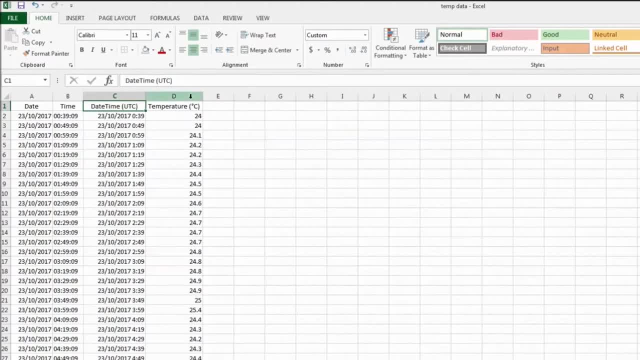 that's UTC. we need to convert them into Australian Eastern Standard Time, which is UTC plus 10 hours. Create a new column and type in date time AEST, And then type 10 hours in a blank cell. Use the formula. 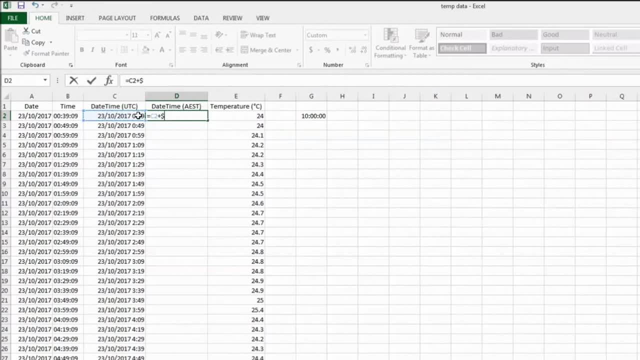 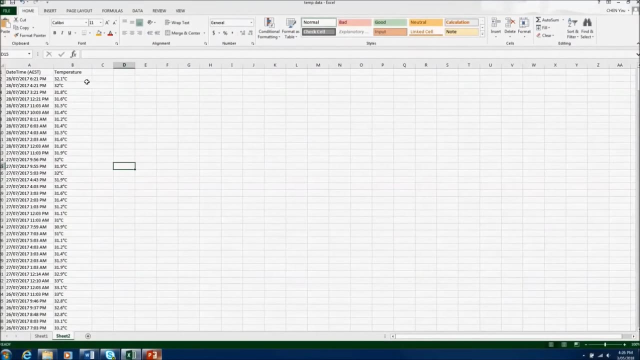 D2 equals C2 plus $G$2.. Use the dollar sign to lock the cell and apply the formula for the whole column. If the data has degree C on the end of the temperature, Excel will think it is at tax entry and won't graph it properly. 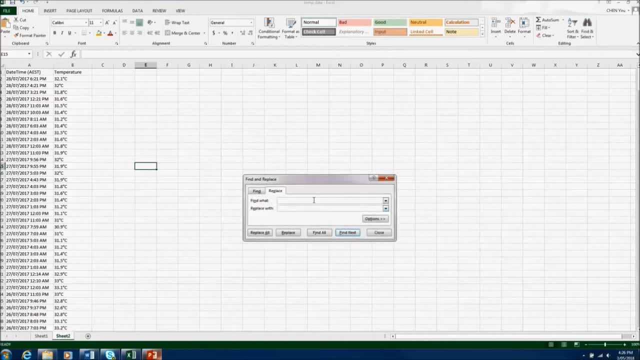 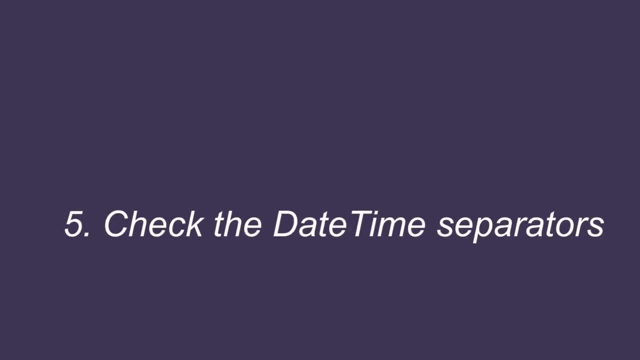 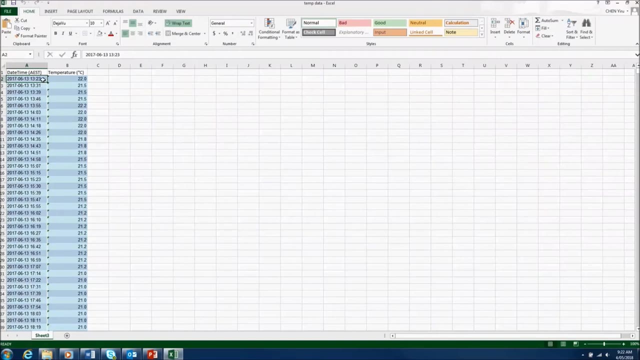 Use find and replace function To replace the degree C symbol with blank. Some datum data use dash as the separator. We need to use find and replace function to replace all dash with slash. Make sure that Excel recognizes that datum format. Okay, In some data file we can see there are green triangle on top left of temperature data cells. 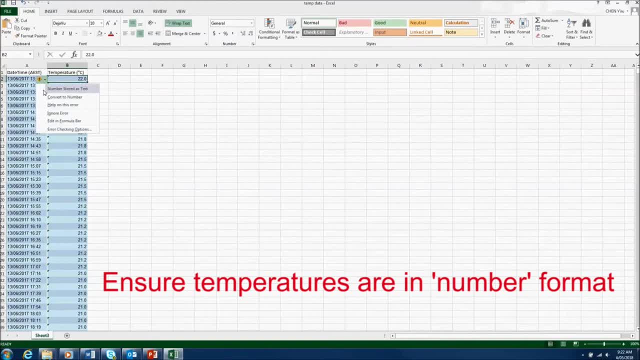 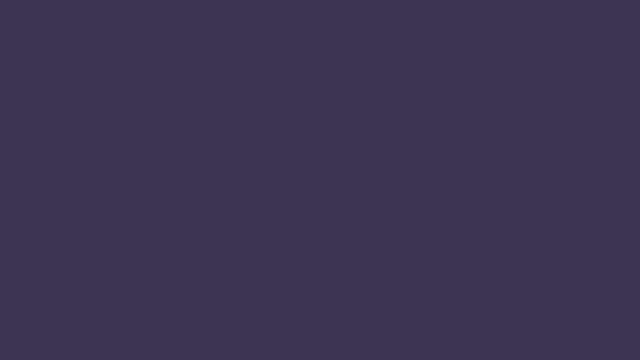 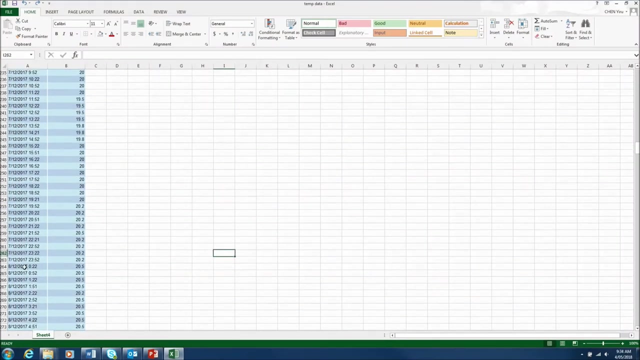 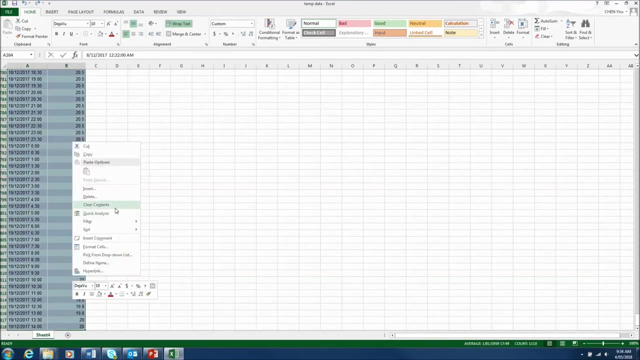 This means those numbers are stored as tax. We should convert them into numbers. We can do this quickly by clicking tax to columns under data menu and finish. Before graphing. we should delete data that recorded before and after the logger was inserted. Please find out this information from supply chain partners. whoever inserted and removed. 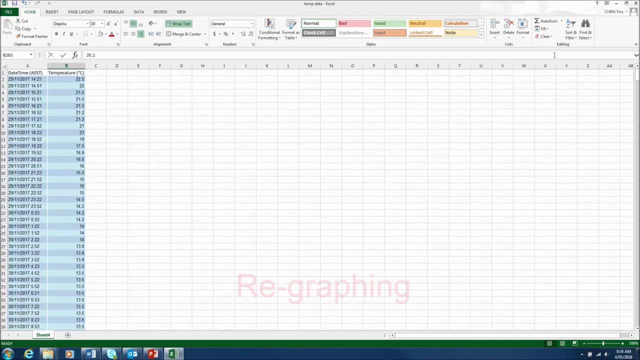 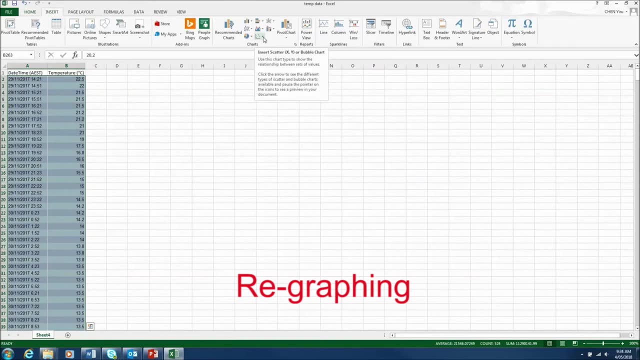 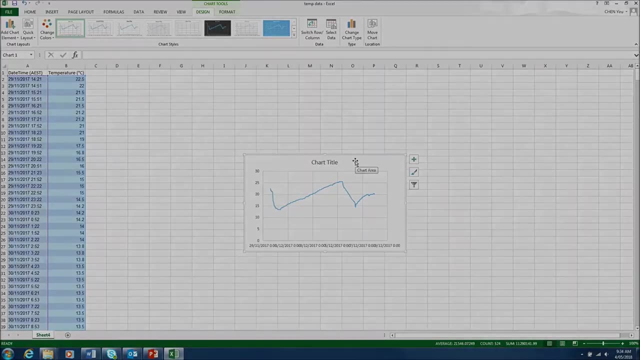 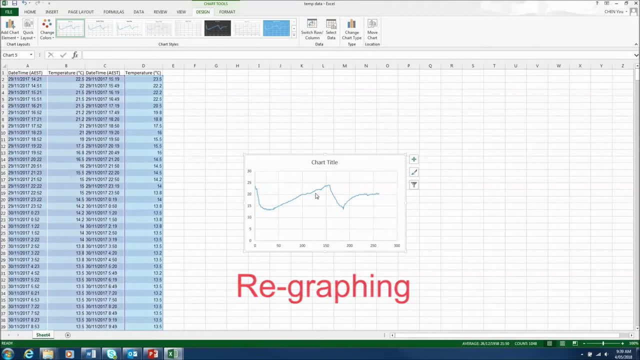 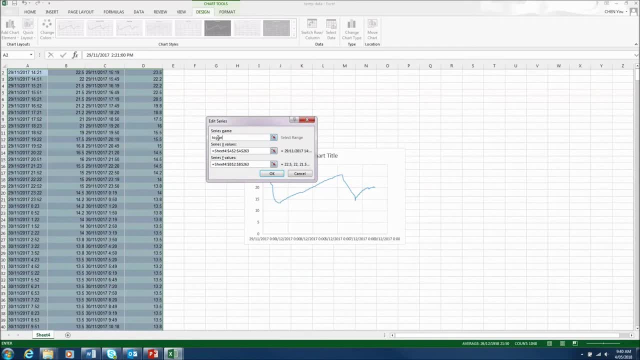 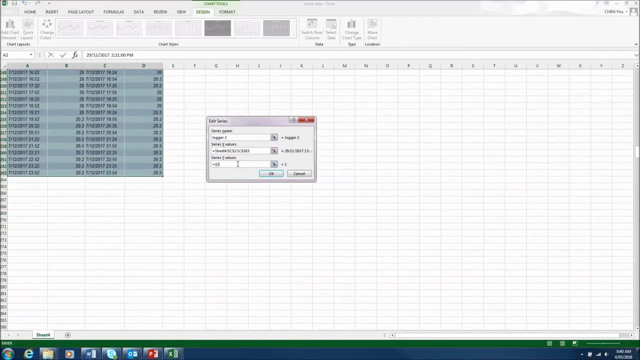 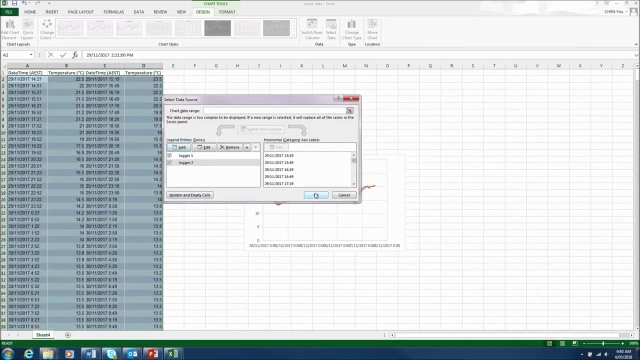 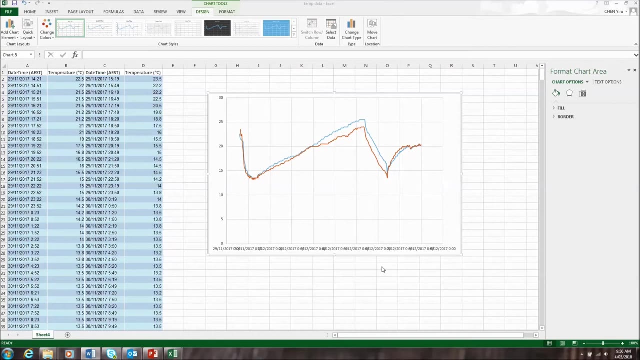 And select relevant data to be graphed. Click OK. For better layout, we need to trim the start, end and intervals for daytime axis. Double click on graph's horizontal axis. Click the last symbol under Axis Options to adjust maximum and minimum bounce value. 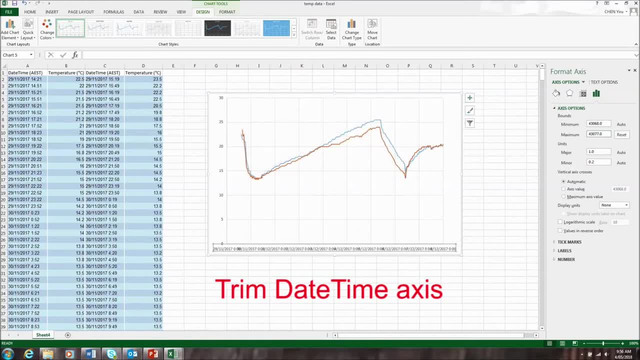 Value 1 here means 1 day. Auto value in Major means the number of days for daytime interval. Auto value in Minor means the number of days for Monday And Auto value in Minor means the number of days for Monday. If we want to make daytime label easier to read, click on graph's horizontal axis. 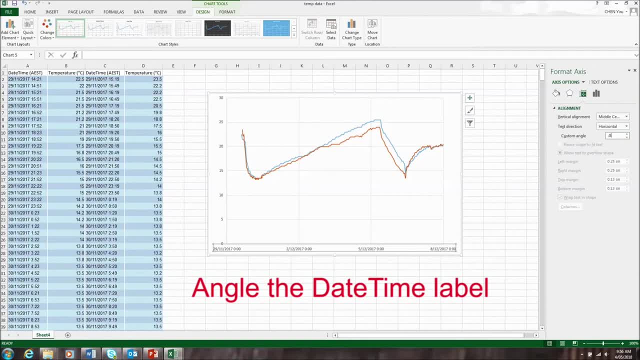 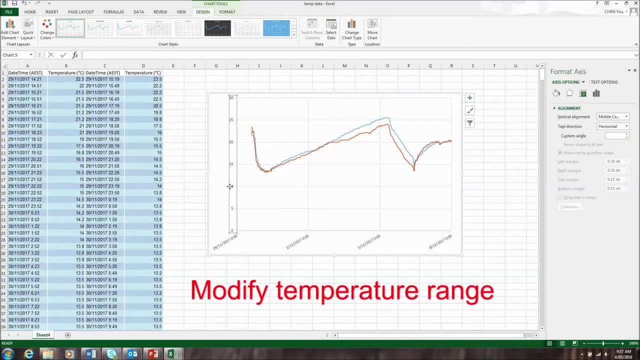 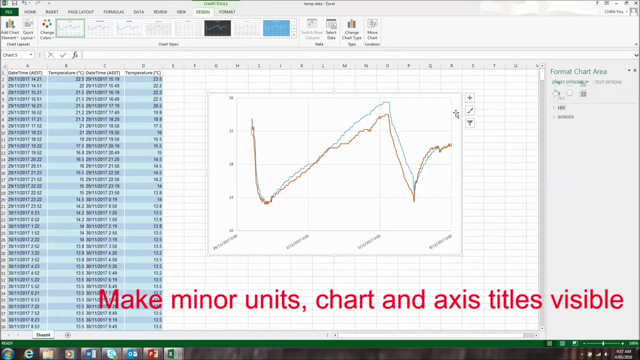 Select the third symbol under Axis Options. Set minus 30 degree for custom angle. Same steps as trimming daytime axis. Adjust bounce and unit's value to trim temperature range appropriately, And that's it. Click on the graph's horizontal axis. Click on the graph's horizontal axis. 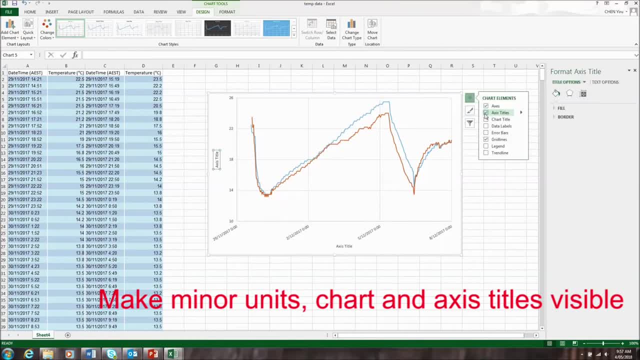 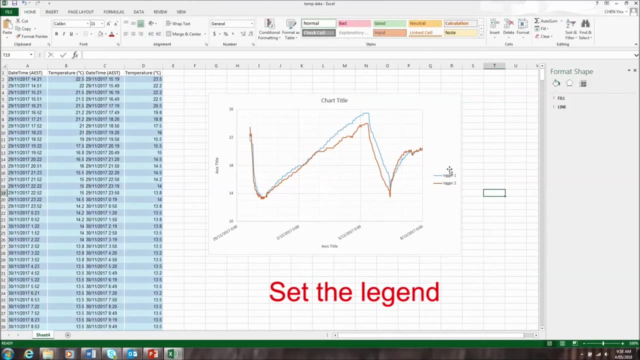 There is a plus symbol on top right corner. Take axis titles and chart titles. Click grid lines and take primary minor horizontal and primary minor vertical. Also, take the legend. We can also change the location legend to bottom, left or top. I prefer to put it at top. 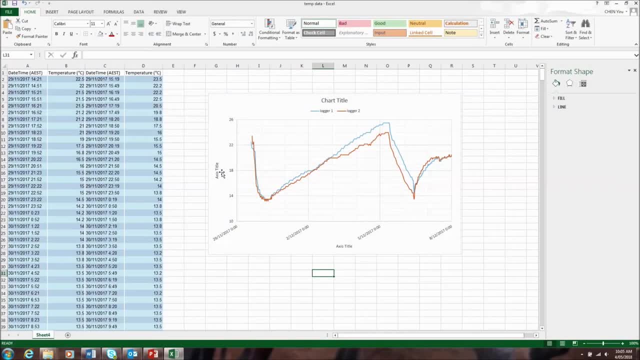 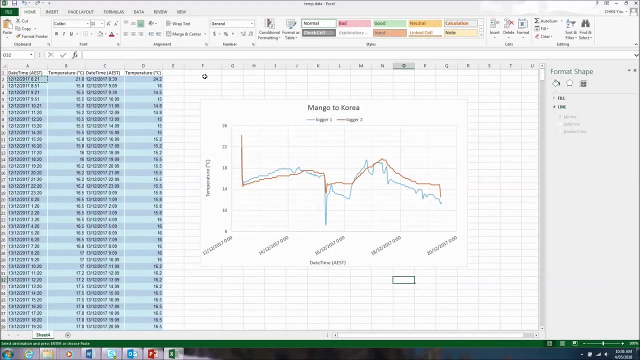 For the vertical axis we call it temperature degree C And for horizontal axis we put daytime. The chart title of this graph could be Mango to Korea. Then adjust font size to make all titles and the legend clear to read. Set up a range with X and Y values in a blank area on the same Excel sheet. 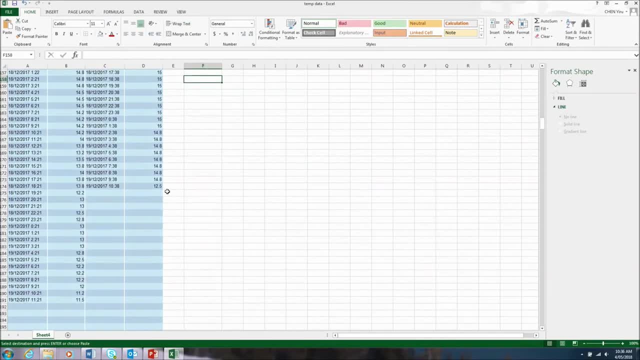 The X value ranges from start to end date of recording. Then we can change the font size. Set up a range with X and Y values in a blank area on the same Excel sheet. Then we can change the font size. Set up a range with X and Y values in a blank area on the same Excel sheet. 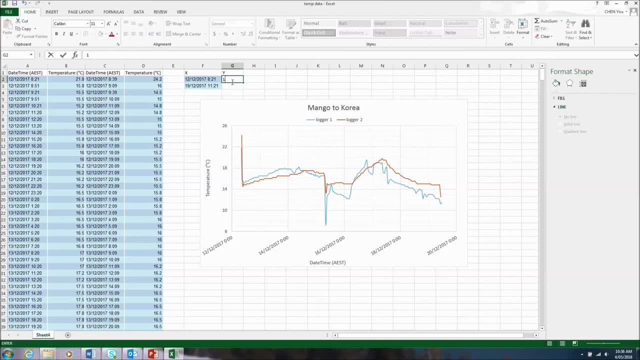 The Y value corresponds to your temperature limit For Mango. we could put 13 degrees here. Then right-click on the graph, choose Select Data and add Type series name and choose X and Y values. We can call it ideal temperature.